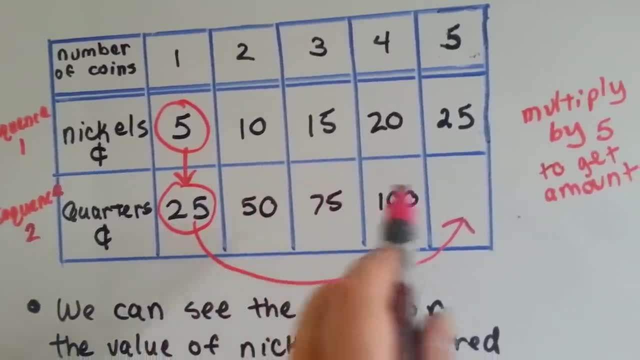 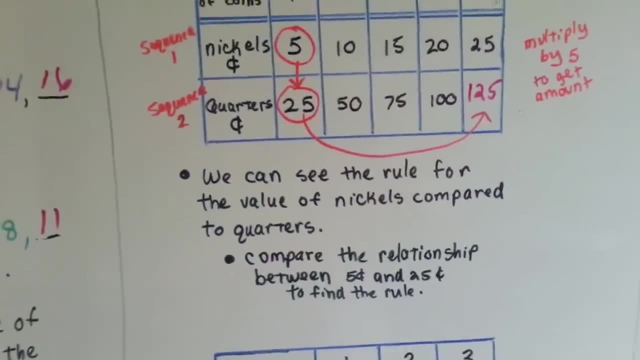 We could also go up by 25 here, because, look, it keeps going up by 25.. So if you say 125, should go here. you're right, See, We compared the relationship between the nickels and the quarters and we saw what the sequences were doing in relationship to each other. 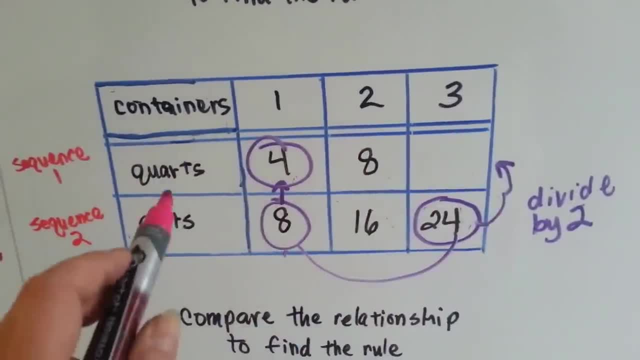 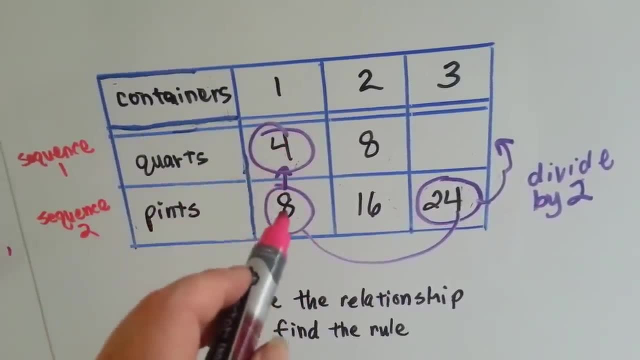 Well, if we had numbers of containers, and in sequence 1 we had how many quarts were in the container and sequence 2 were how many pints, 4 quarts would be 8 pints. 8 quarts would be 16. 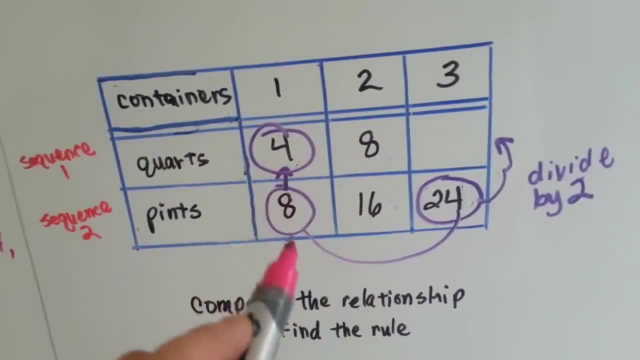 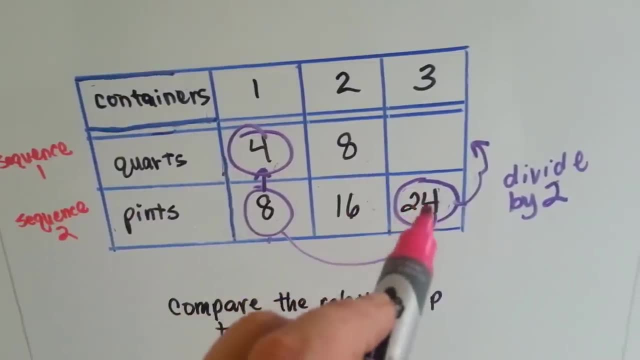 pints. Do you see the relationship of what's happening between quarts and pints? 8 divided by 2 is 4,. 16 divided by 2 is 8, so that means 24 divided by 2 would be 12,. 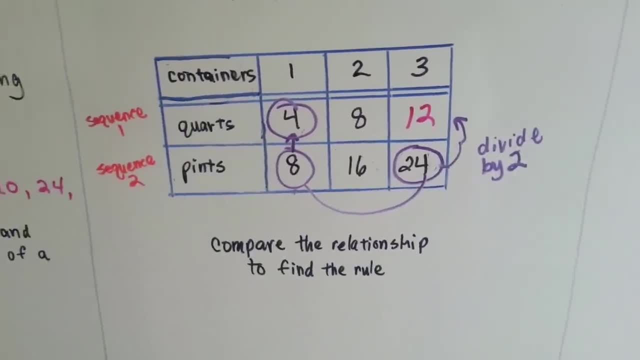 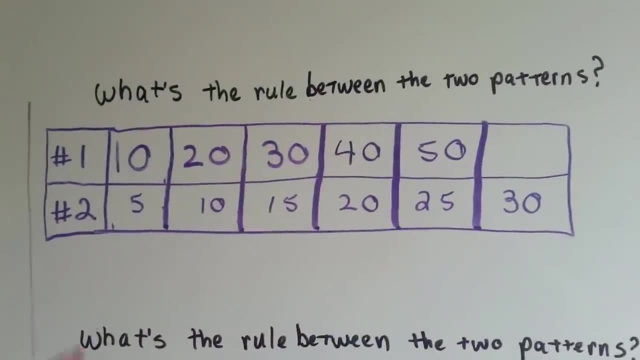 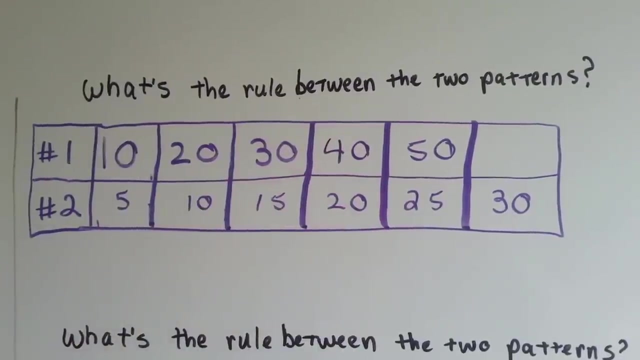 and we'd be able to figure out what the missing number is. So we compare the relationship to find the rule. What's the rule between these two patterns? Can you tell 10 and 5, 20 and 10, 30 and 15,, 40 and 20,, 50 and 25.. If you say the number 2, see if you can tell. 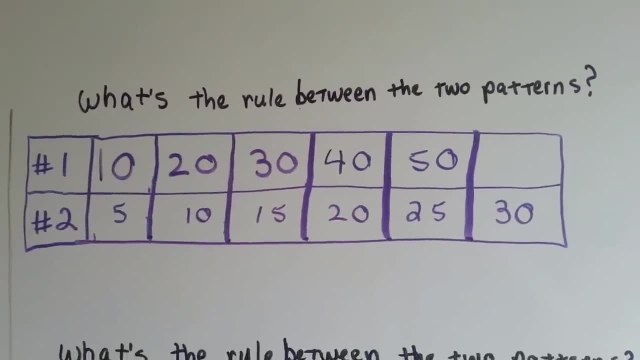 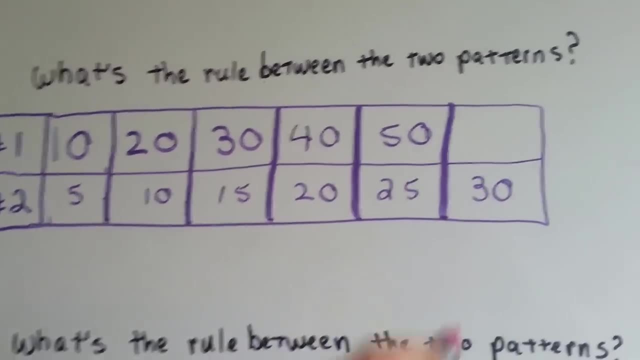 that the sequence is half of what the number 1 ones are. you're right. So do you know what would go there If these are half and these are going up by 10s, aren't they? So if you said 60,? 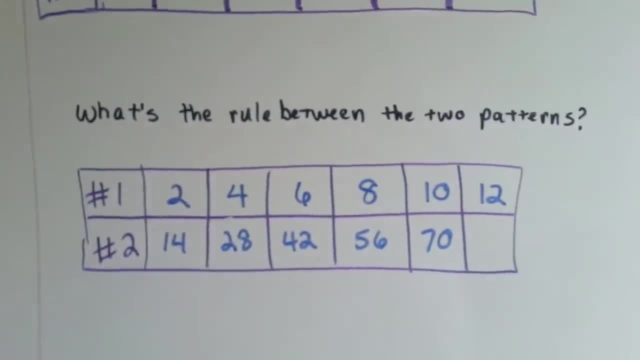 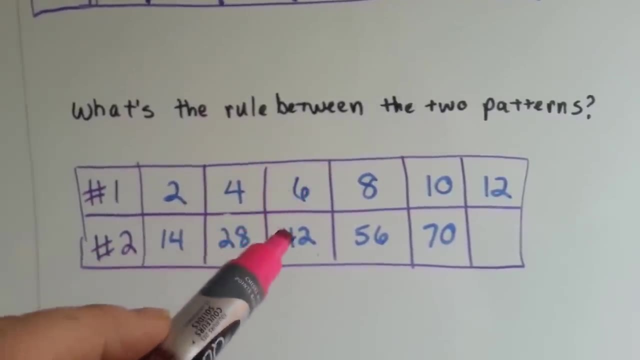 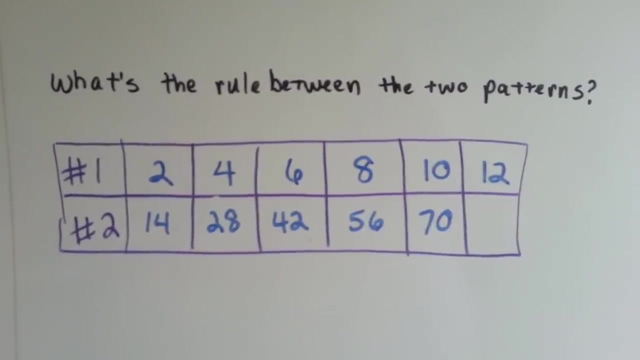 you're right. See How about this one. What's the rule between the two patterns? 2 and 14,, 4 and 28,, 6 and 42,, 8 and 56,, 10 and 70.. Can you see the relationship between the two patterns? 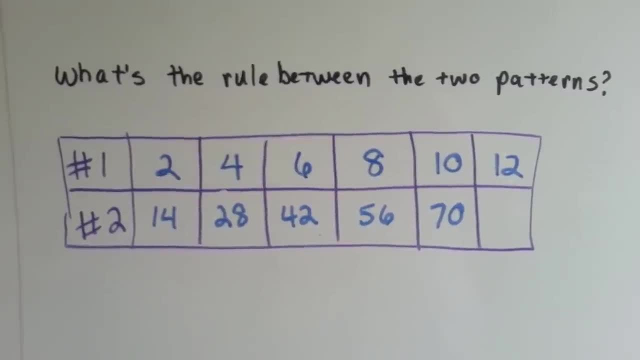 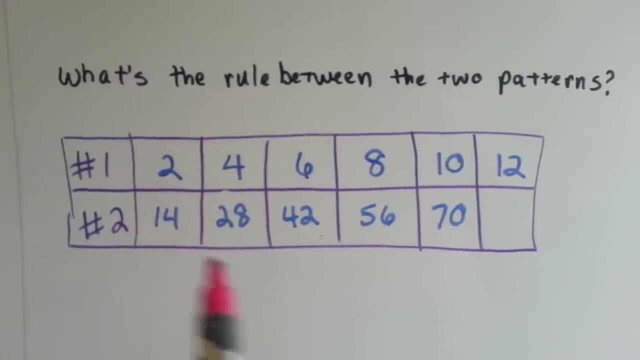 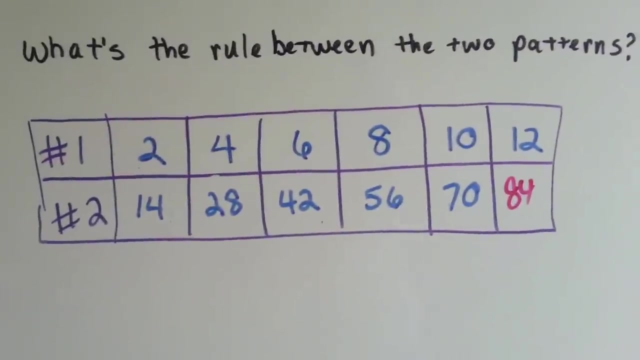 This one's a little harder. The 10 and 70 might help you, But if you know your times table, if you said they're multiplied by 7, you're right. So if we multiply 12 times 7, we'll get 84, and we'll have the missing number, See Sequence. number 2 was 7 times more than. 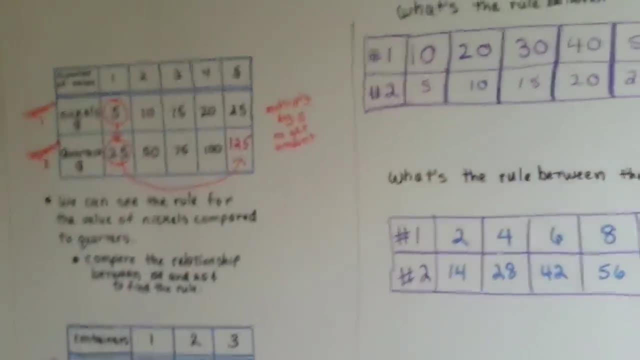 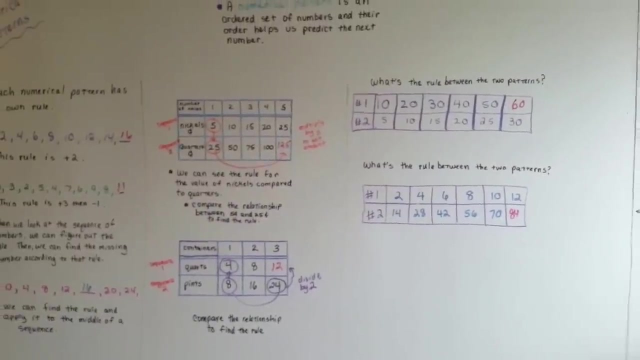 the numbers that were in sequence number 1.. See, So we can find the relationship between the two patterns and then we can fill in the empty space. We can find the rule for the sequence and we'll be able to fill in the empty space. 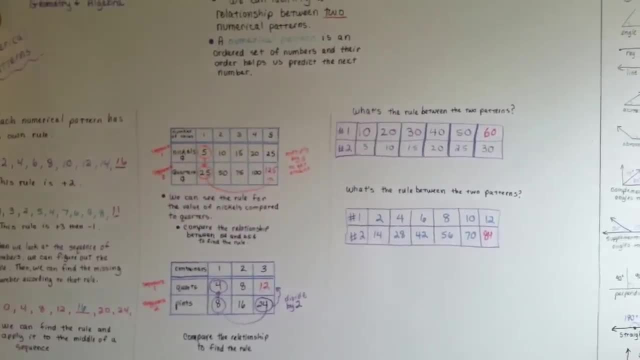 See. So those are numerical patterns. I'll see you next video. Bye. 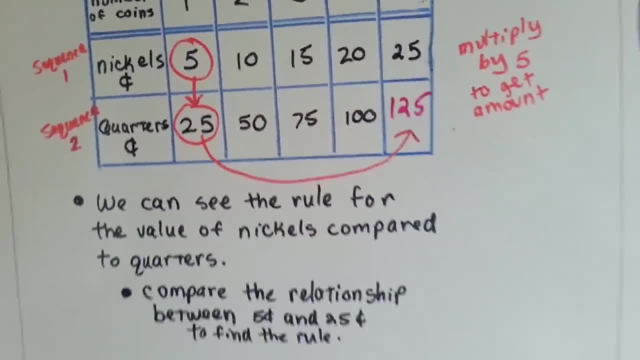 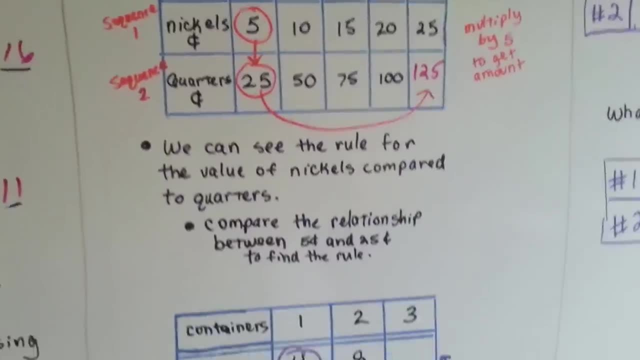 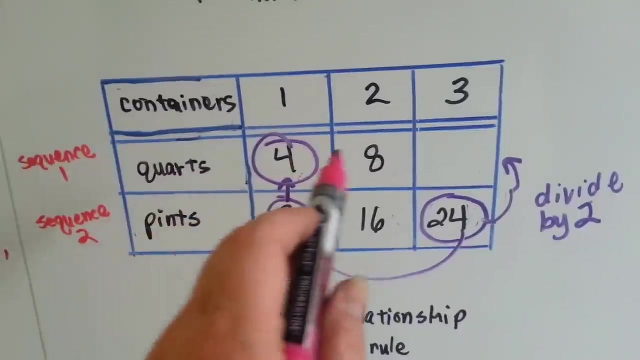 So if you say 125. You should go here. you're right. See, We compared the relationship between the nickels and the quarters and we saw what the sequences were doing in relationship to each other. Well, if we had numbers of containers, and in sequence 1 we had how many quarts were in the container and in sequence 2 were how many pints. 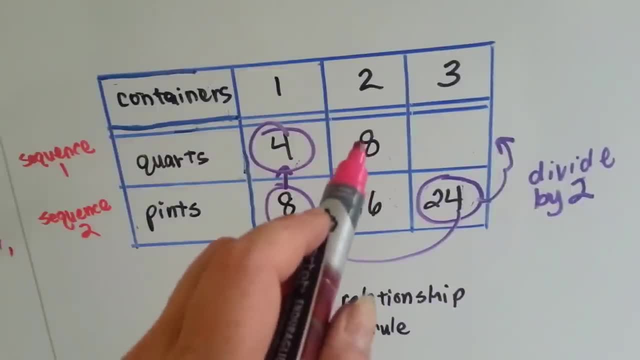 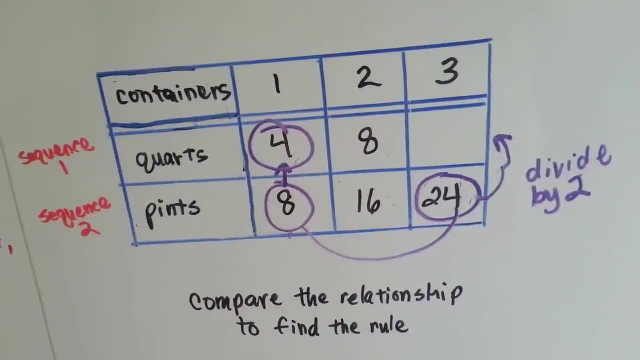 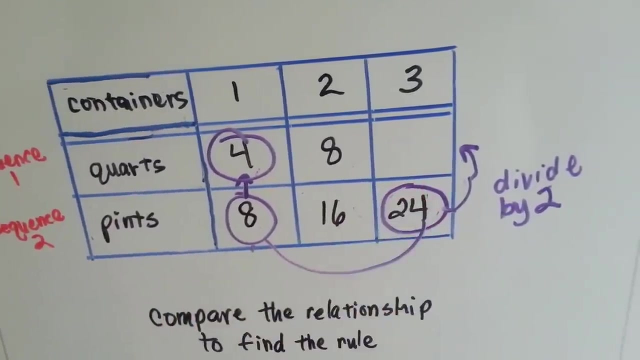 4 quarts would be 8 pints. 8 quarts would be 16 pints. Do you see the relationship of what's happening between quarts and pints? 8 divided by 2 is 4,. 16 divided by 2 is 8.. So that means 24 divided by 2 would be: 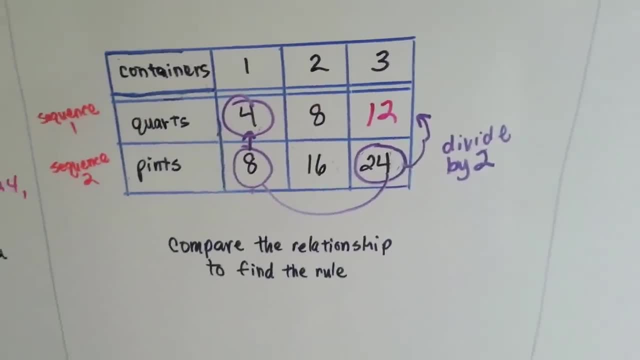 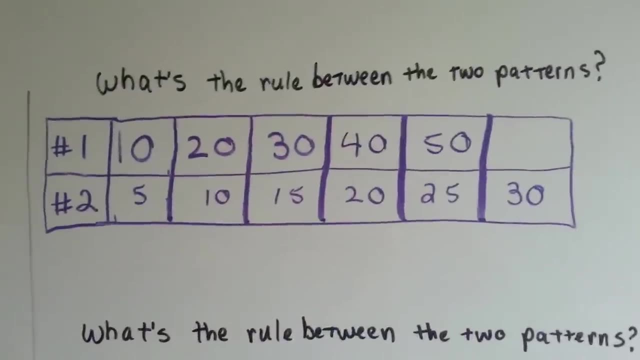 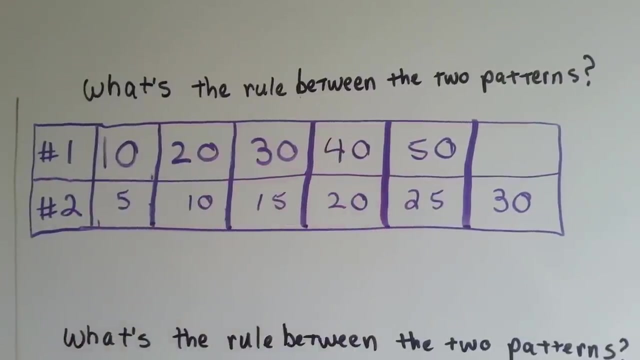 12. And we'd be able to figure out what the missing number is. So we compare the relationship to find the rule. What's the rule between these two patterns? Can you tell: 10 and 5, 20 and 10, 30 and 15, 40 and 20,, 50 and 25.. 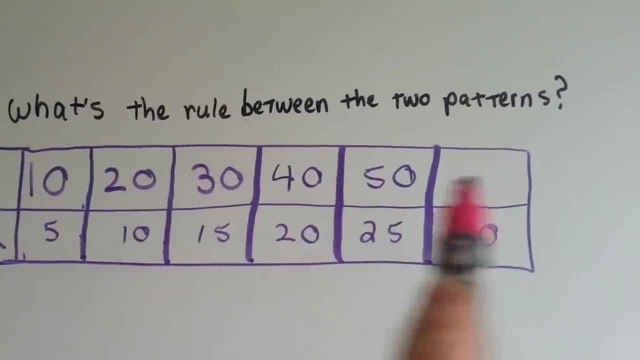 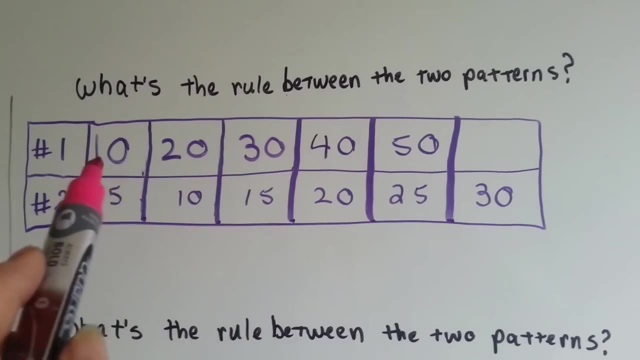 If you say that number 2, is half of what the number one ones are, you're right. So do you know what would go there if these are half? And these are going up by tens, aren't they? So if you said 60,, you're right. 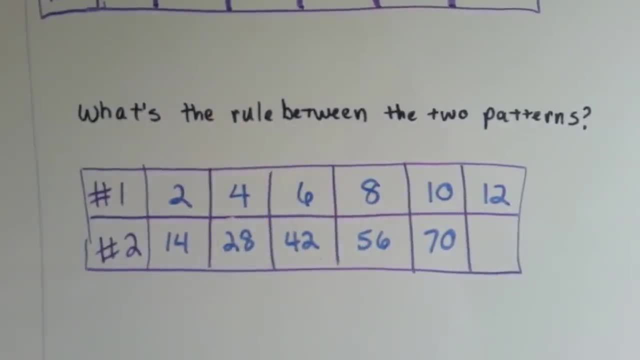 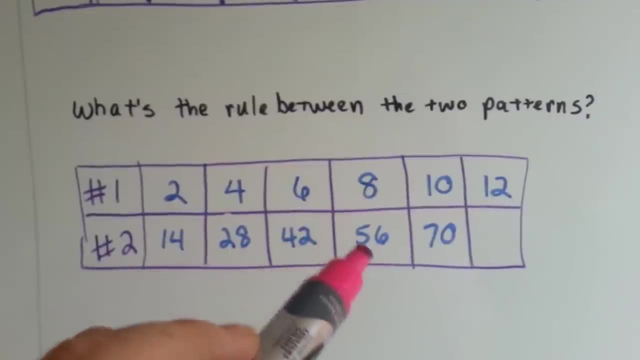 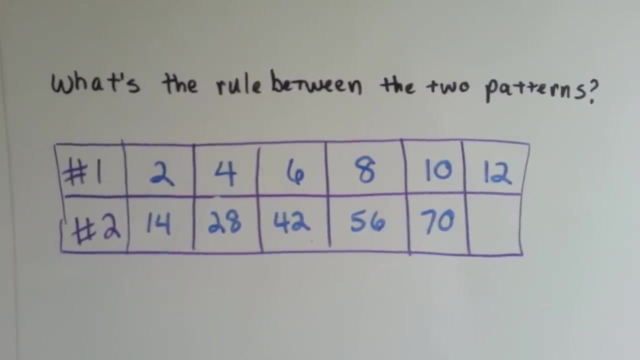 See How. about this one? What's the rule between the two patterns 2 and 14,, 4 and 28,, 6 and 42,, 8 and 56,, 10 and 70.. Can you see the relationship between the two of them? 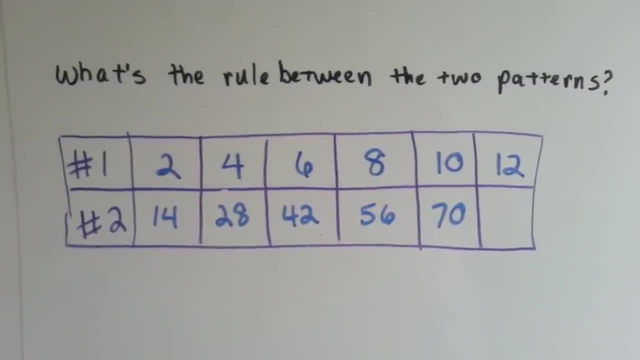 This one's a little harder. The 10 and 70 might help you, But if you know your times table, if you said they're multiplied by 7, you're right. So if we multiply 12 times 7, we'll get 84,. 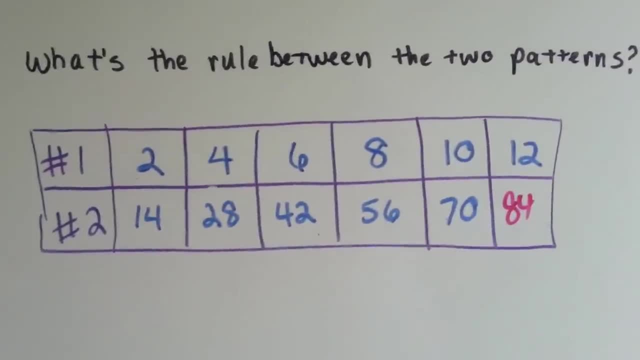 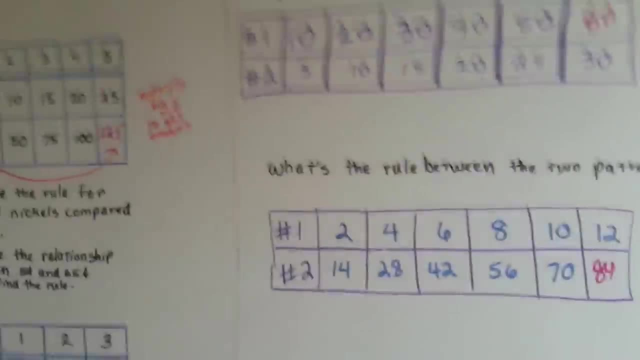 and we'll have the missing number. See Sequence number 2 was 7 times more than the numbers that were in sequence number 1.. See, So we can find the relationship between the two patterns and then we can fill in the empty space. 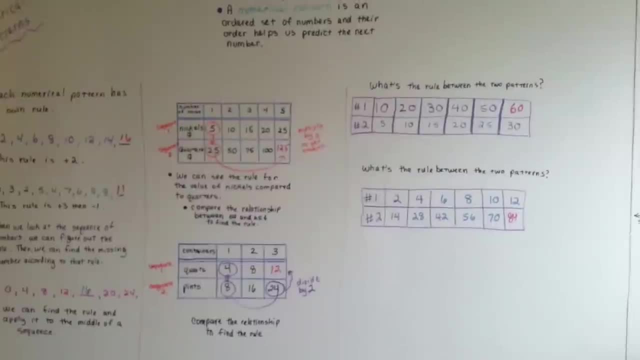 We can find the rule for the sequence and we'll be able to fill in the empty space. See So, those are numerical patterns. I'll see you next video. Bye.